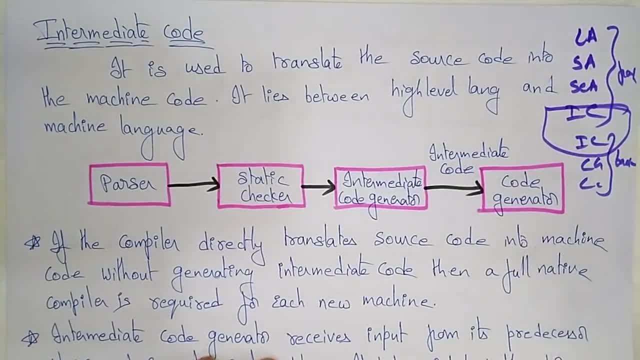 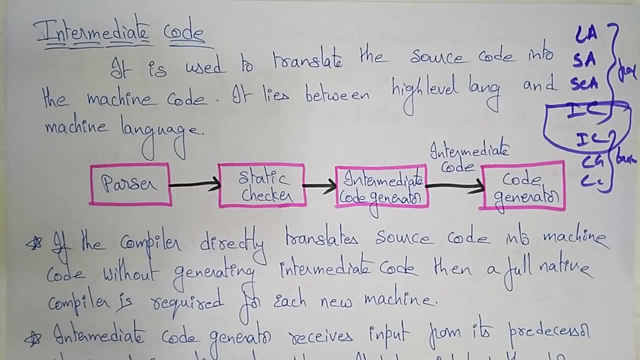 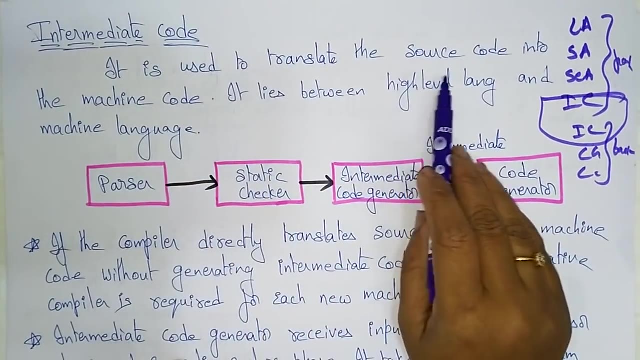 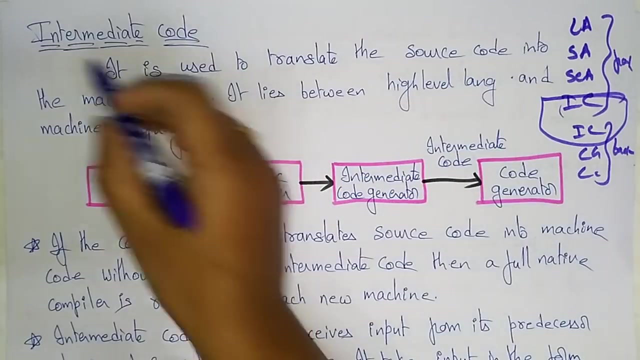 So far we have seen the lexical analyzer, syntax analyzer, and semantics is just representation of the means. It's a semantic rules we discussed in the syntax directory. Now let's see intermediate code. It is used to translate the source code into a machine code. The main concept of intermediate- the name itself is saying it is an intermediate Acts in between, from source to destination. 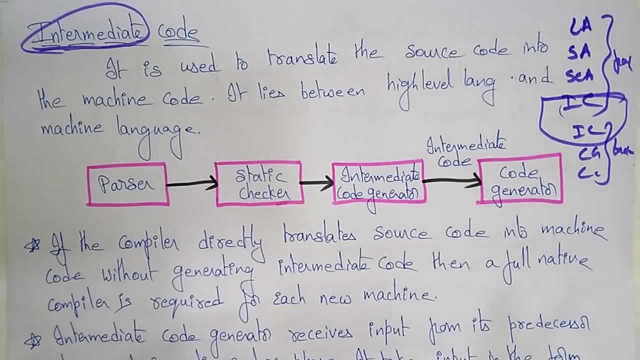 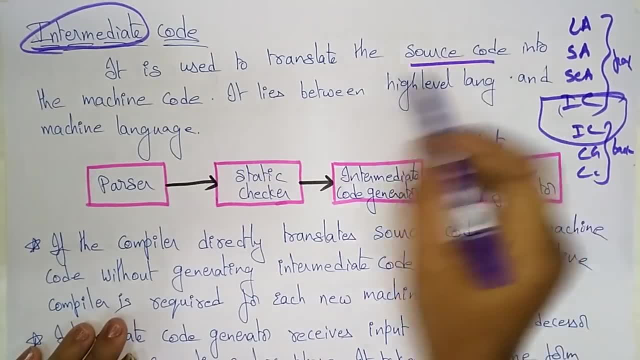 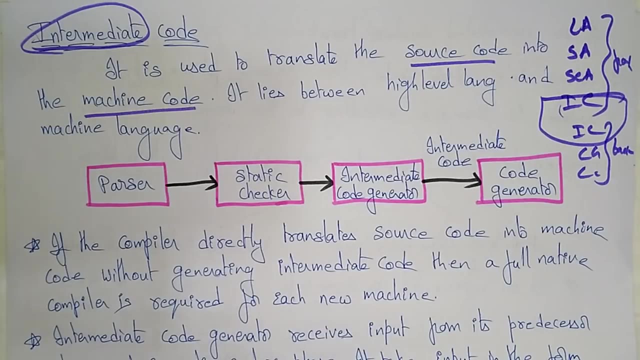 If you want to reach from source to destination, there is a mediator, is there That is an intermediate, So it is from between the source and the destination. That is a source code. So you can use this as an intermediate code or you can take it as an assembly code. Means the compiler will give the result as an assembly code. Okay, So it is used to translate the source code into the machine code, which is an assembly language. 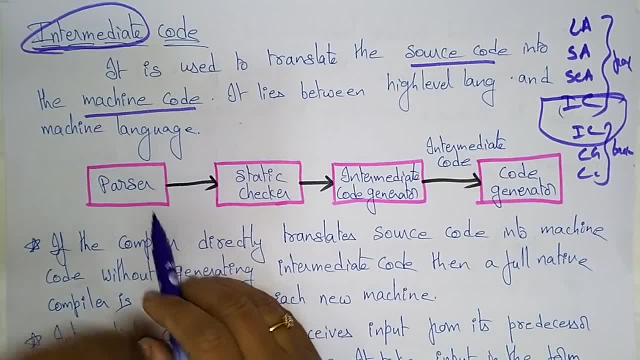 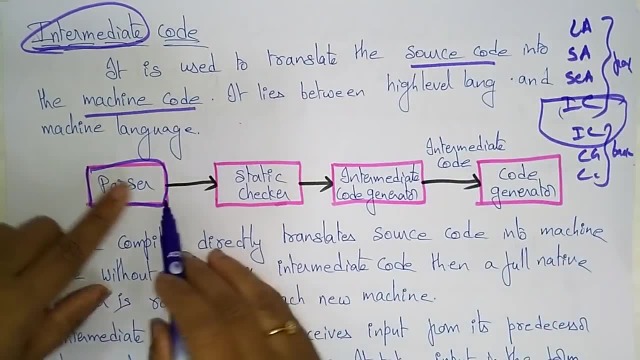 It lies between the high level language and machine language. So let's take this is a parser. Okay, You know that the parser is that represented as a syntax analyzer. Okay, So parser is first static. checker will be there with the help of the semantic analyzer. 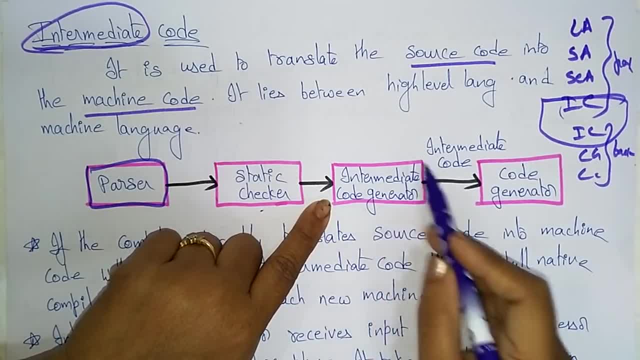 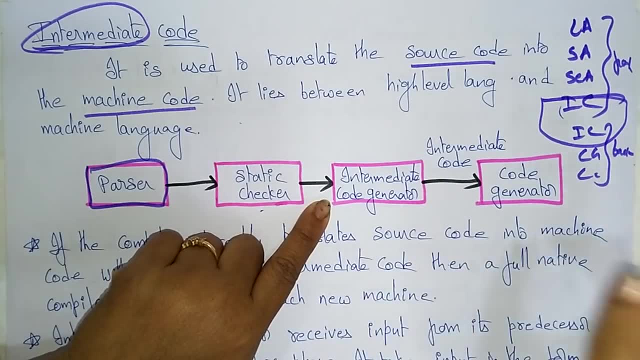 Next you have the semantic analyzer. So you have the semantic analyzer. Next you have the semantic analyzer is the intermediate code generator. So this intermediate code generator is going to give the already converted information to the code generator with the help of the intermediate. 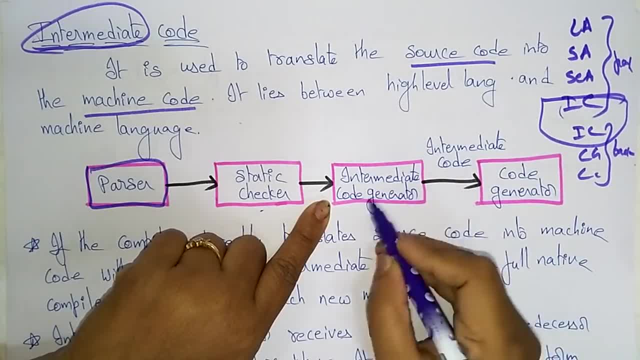 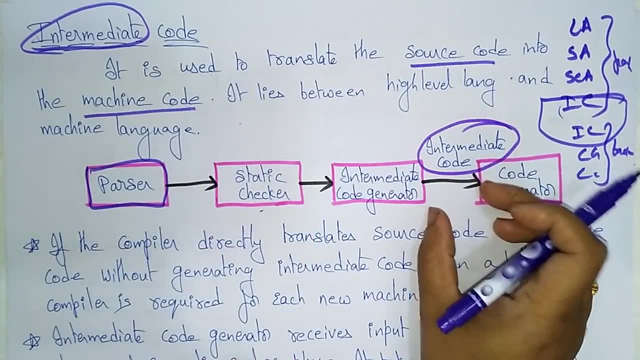 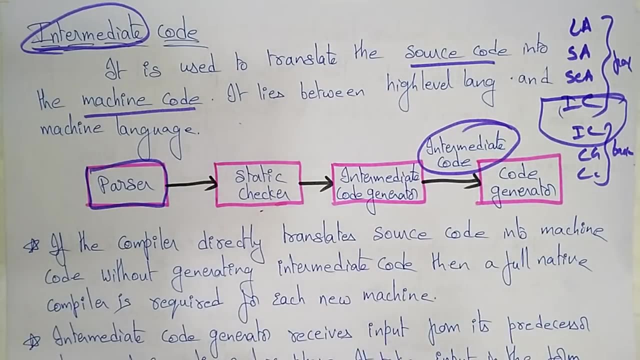 code. So, ok, So the intermediate code generator is generating intermediate code to the code generator. So this intermediate code consisting of what the compiler wants means already it is in the form of a readable format of the code generator. ok, So it is almost readable by the 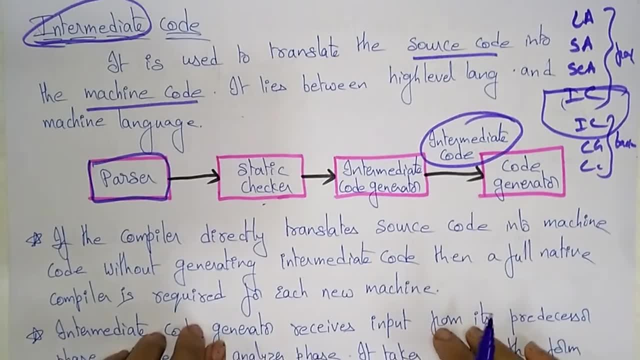 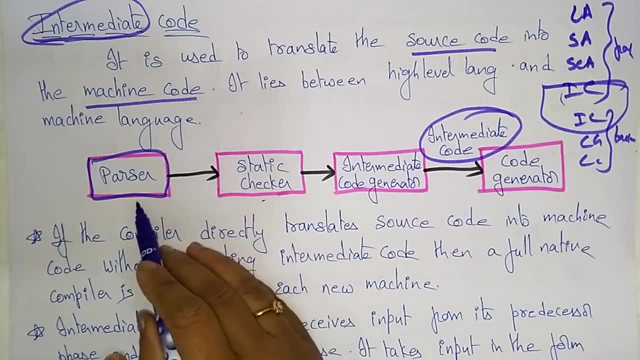 destination. ok, that is a target language. So if the compiler directly translate the source code into machine code? let us take if the compiler is going to directly transfer from source to the destination. So if the compiler directly translate the source code into machine? 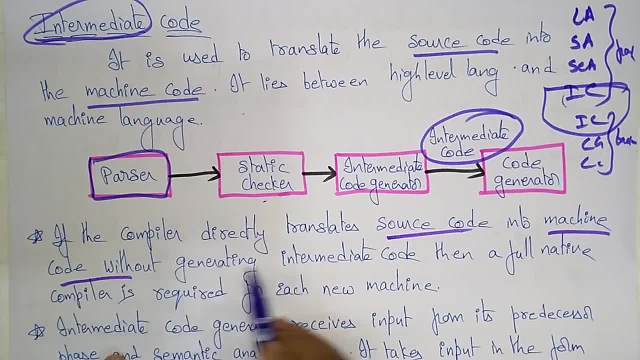 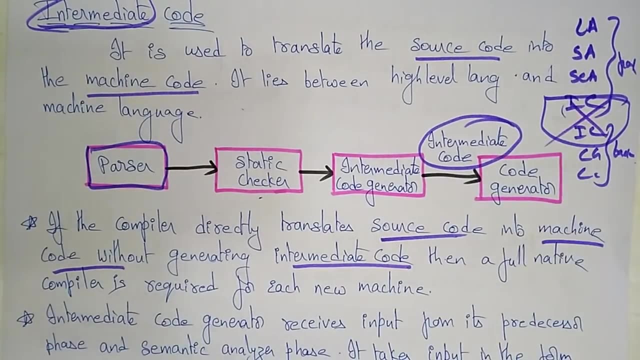 code without intermediate code, then a full native compiler is required for each new machine. So whenever there is no requirement for the- if you are not introduced- intermediate code, let us take suppose there is no intermediate code in the compiler. So then what it is doing? 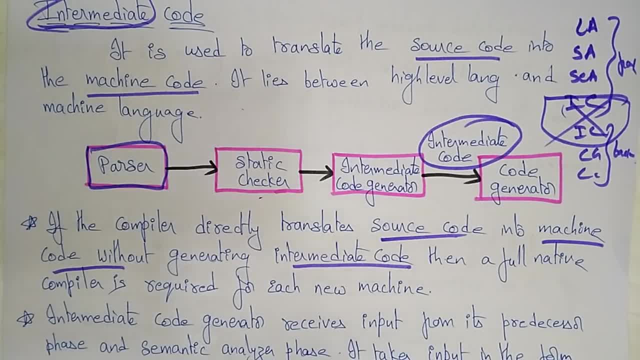 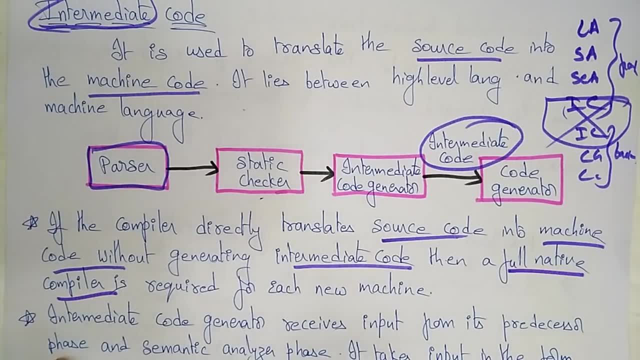 So for whatever the new machines, whatever the machines you are taking, for each and every machine there should be a full native compiler is required, For each and every machine, So, ok, So if the compiler is doesn't having intermediate code, 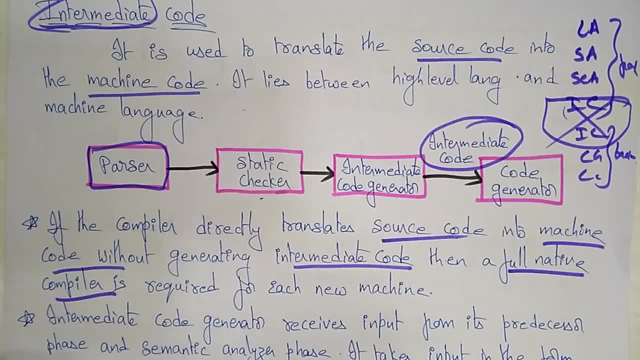 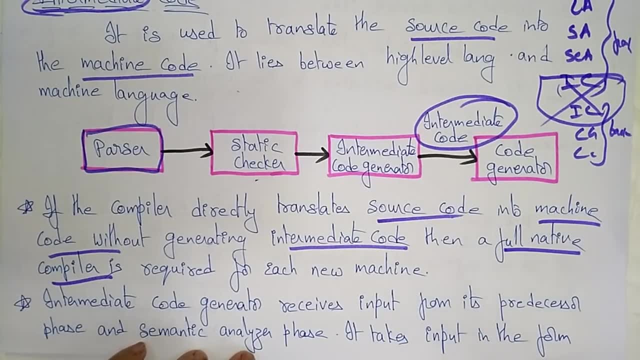 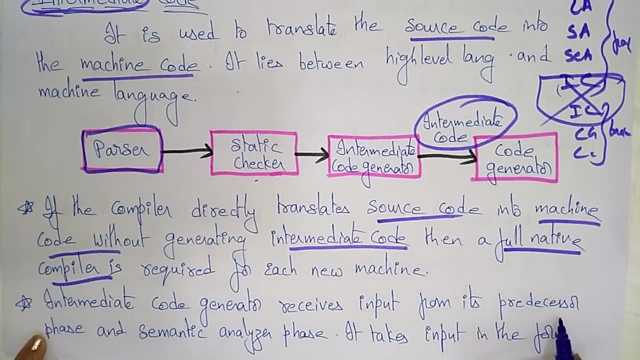 generator, then for each and every machine a full native compiler is required. Otherwise there is no multiple compilers are not required for each and every machine. if there is an intermediate code. Intermediate code generator receives input from its predecessors fees and semantic analyzer fees. So we know that. So if the intermediate code generator receives input from its 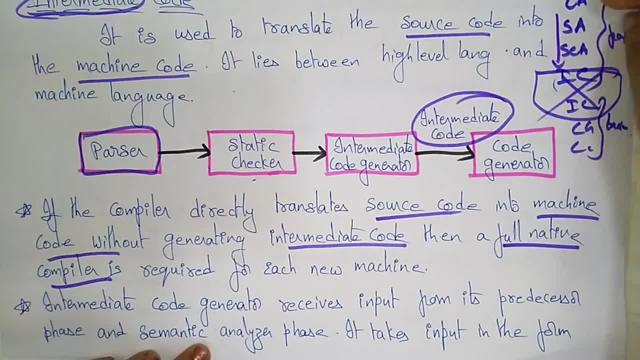 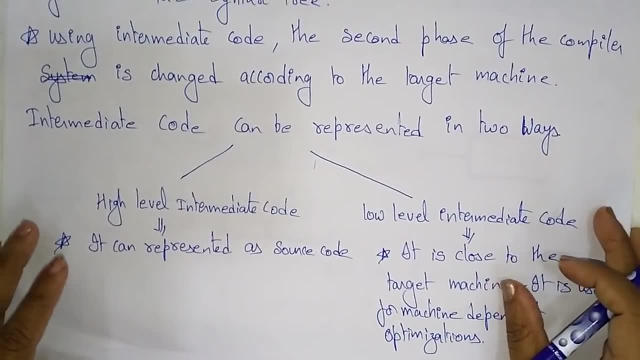 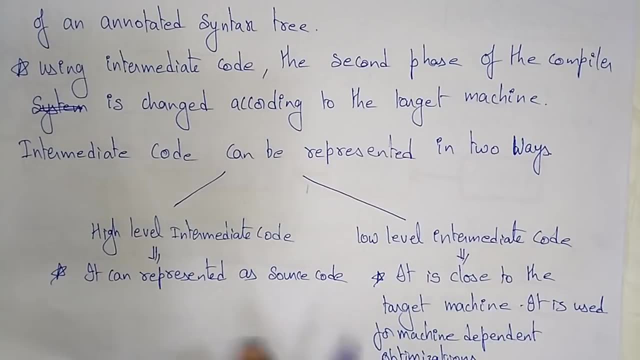 So this intermediate code is going to receive the information from the predeserved faces. It takes input in the form of annotated syntax tree. So all the intermediate code will take the input as a syntax tree because whatever the lexical analyzer- lexical analyzers- is taking the tokens, 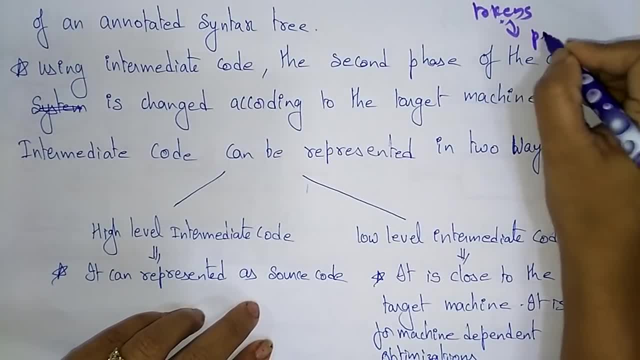 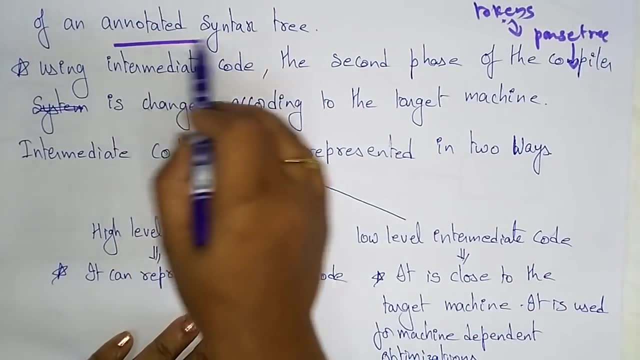 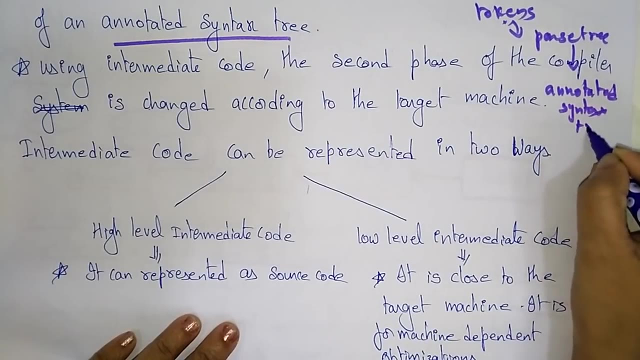 The tokens are converted, represented in the form of parse tree. Okay, so the parse tree is going to be converted in the semantic with the help of the semantic rules, with like annotated, annotated syntax tree, So that I will explain now what is this annotated syntax tree? 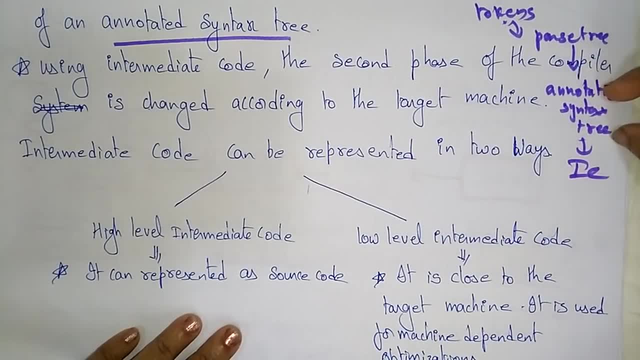 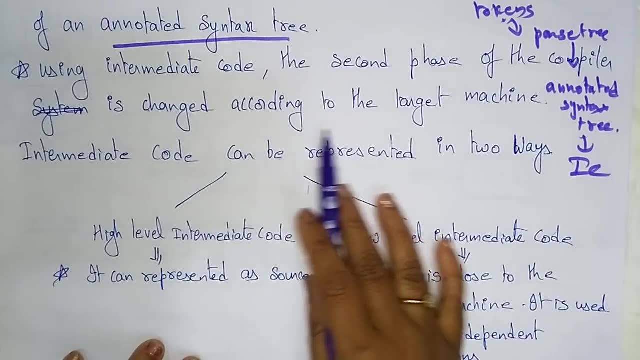 Okay, so then the intermediate code will take the input as annotated syntax tree. Using intermediate code, the second phase of the compiler is changed according to the target machine, So that I said now. So intermediate code can be represented in two ways. 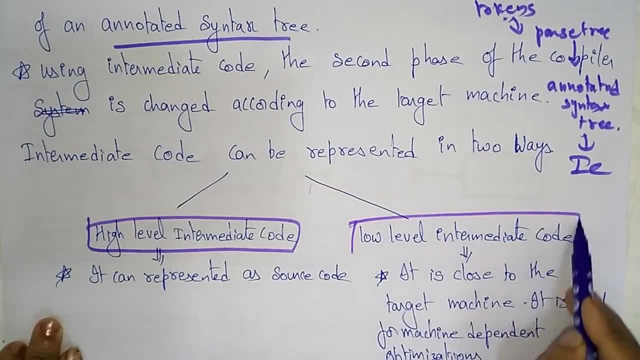 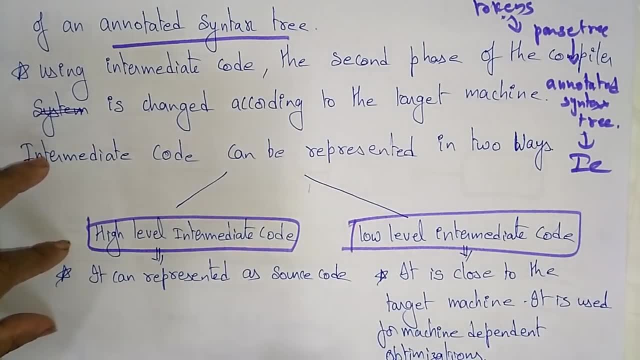 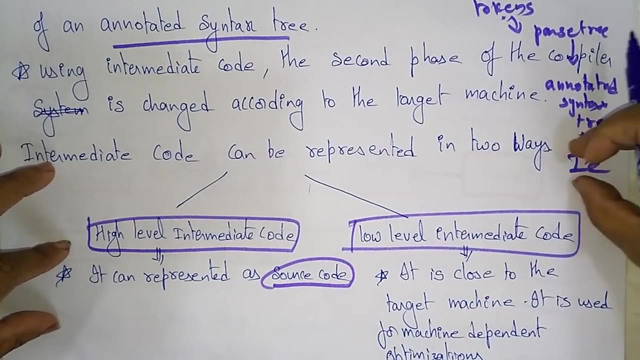 One is a high level intermediate code and another is a low level intermediate code. So you can represent the intermediate code as high level and the low level. High level is nothing, but it can represent it as a source code. So whatever the data that you are taking, that data is taken by the intermediate code is at the source code. 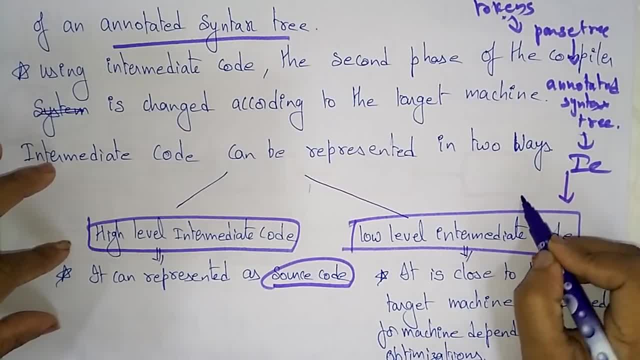 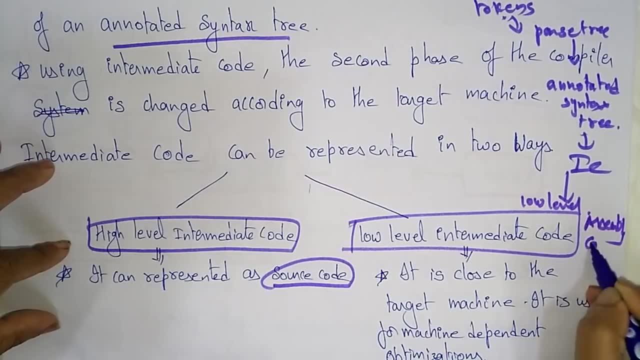 That is a high level. So whenever it is coming down it reaches to the low level Because it has to reach the assembly code. It has to convert the data into assembly code. So that is a low level. So from high level to low level.